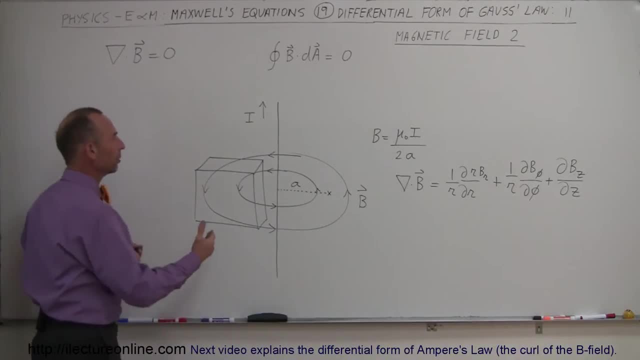 and we're going to use the Gauss's Law for Magnetism. and here again, what we're doing is what we're. if we take the integral form, we can say that it's simply equal to the strength of the B field. okay, that would be determined by this times the area. and you can see that, because of the symmetry if the B field 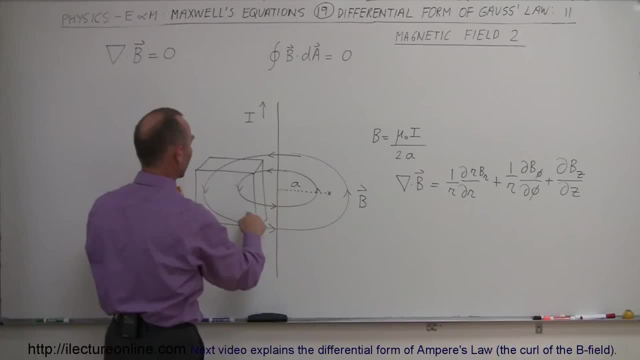 goes through the surface like this, the same amount of B field versus area will travel in the back of the box as comes. come out the front of the box and you see that the net result is that we have so much flux going in, so much flux to come out, and so, therefore, 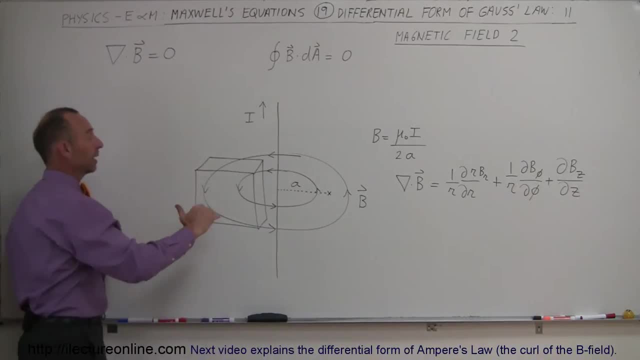 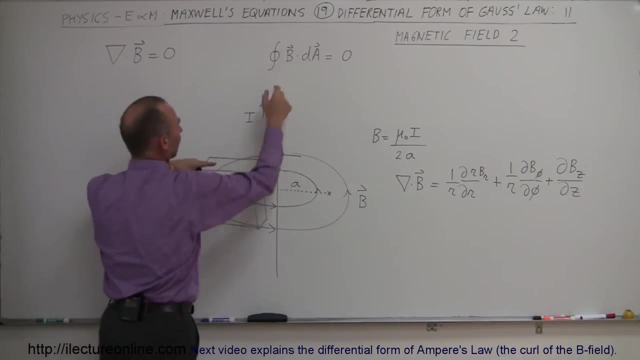 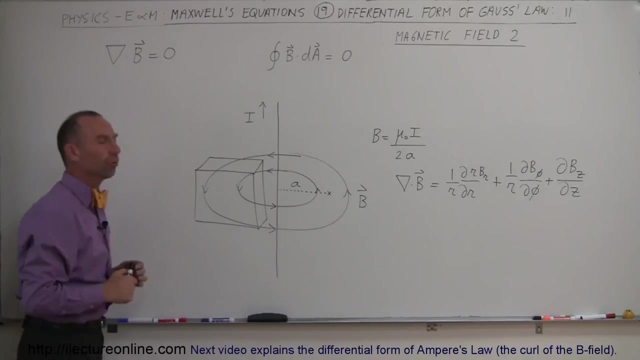 The integral of that should have with would be 0, because in this case the B field is is per is in the opposite direction to the vector of the surface and on the other side it's in the same direction. so the two sides will simply cancel each other out and end up with a 0 on the integral form. but 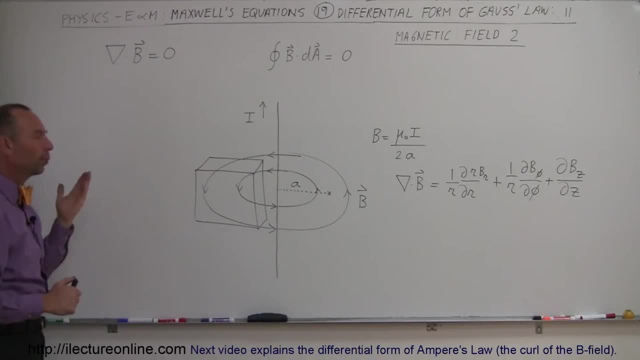 how's that compared to the, to the differential form? well, one way to do it is simply take the divergence in circle coordinates. now, in this case we're in cylindrical coordinates. in cylindrical coordinates because you know you can take it. This has a cylinder in the B field forming a cylinder around the current right here around the wire, the. 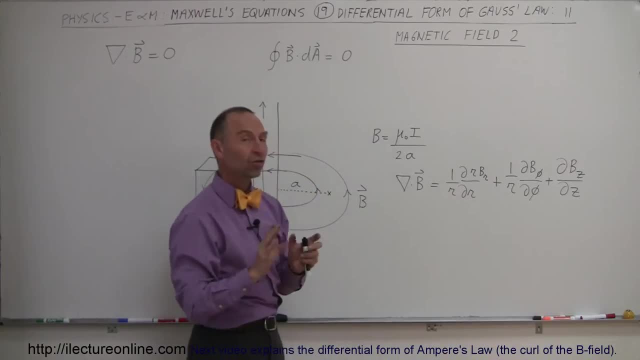 divergence equal to this equation right here now. notice that there's no variation in angle, so no matter in which direction you face, the B field will always be the same. the only thing that matters is the distance from the wire, and also doesn't matter if you're over here, here, here, here or down here, as long as the 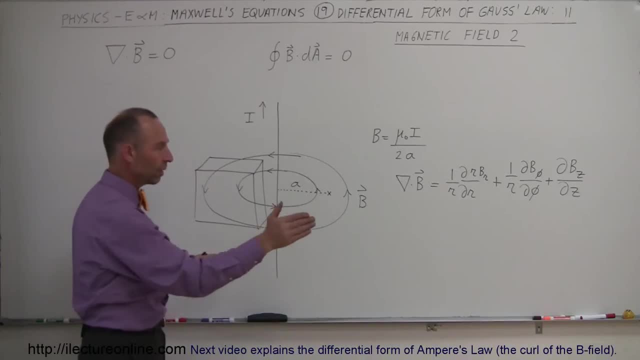 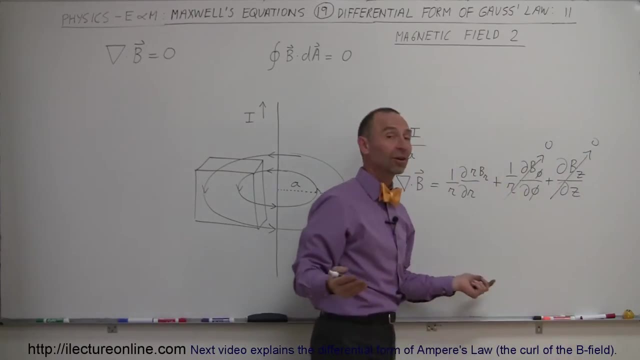 wires long enough. there's no dependency on the Z direction, there's no dependency on angle. so those last two portions of the equation, They become equal to 0 because you take the derivative of that. since they're constant, you get 0. so all we have to do is take the derivative of this. so now, instead of using r, we're going to use the variable a, a being the distance from the wire, and so this becomes 1 over a times, a partial derivative with respect to a of a times this quantity right here, which is mu sub naught times i, divided by 2a. 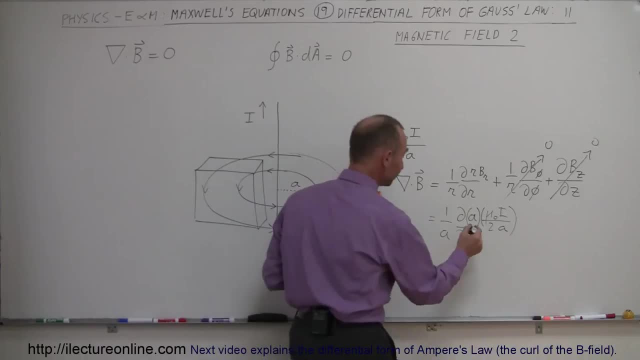 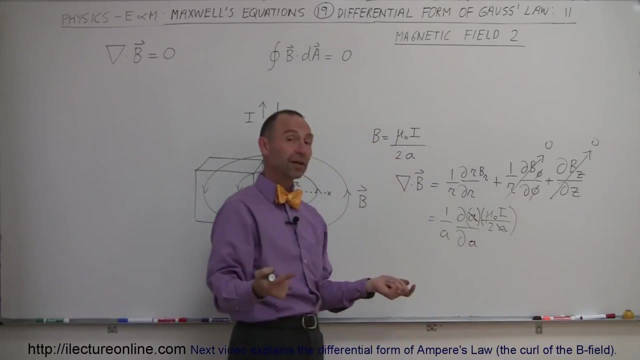 Now this is a derivative of a times this quantity right here, which is mu sub naught times i divided by 2a. Now notice, in this case the a's cancel out and all we're doing now is taking the derivative, with respect to a, of a constant and, of course, taking derivative of a constant equivalent to 0, so this whole thing becomes equal to 0, which is: